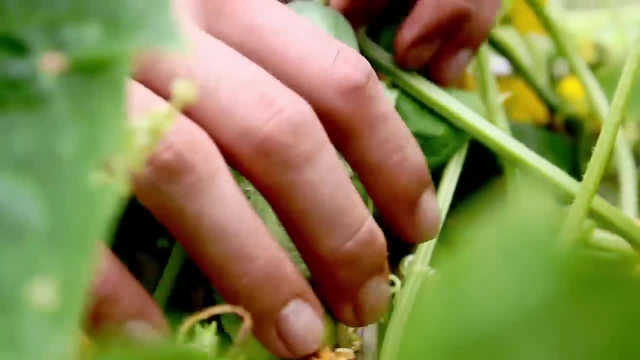 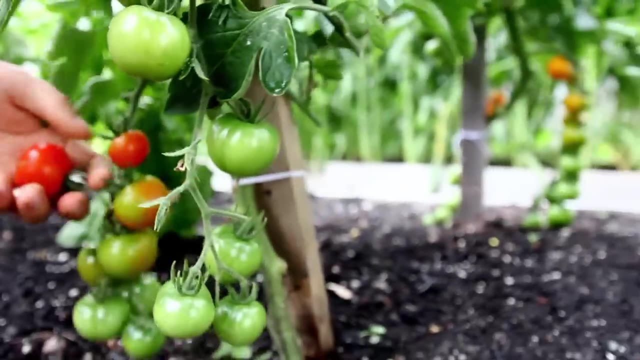 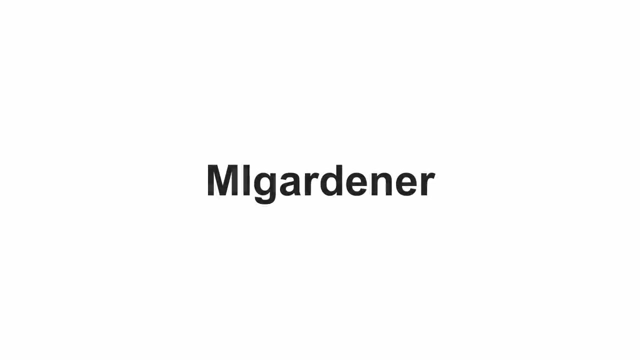 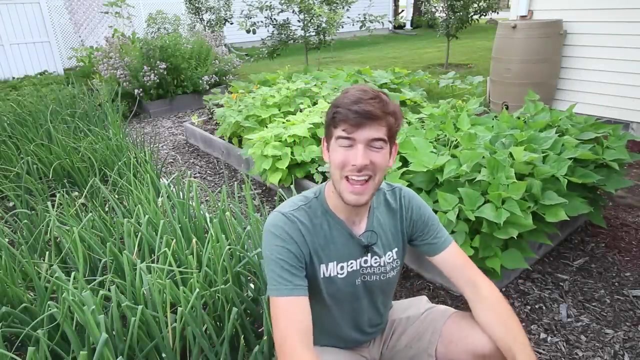 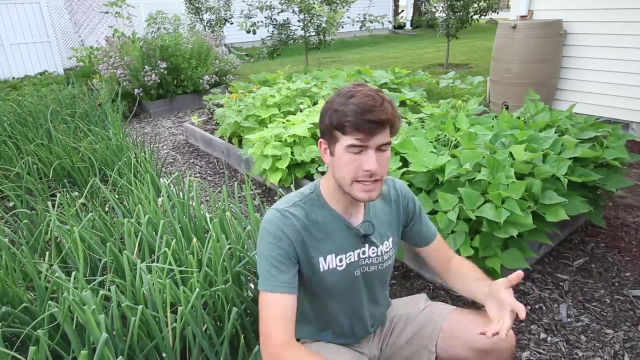 What is going on everyone? Welcome to another very exciting episode right here on the MI Gardener channel. I am so excited about today's video because I'm going to be sharing with you three all-natural pest control methods for ants. Now, ants are something that a lot of people just 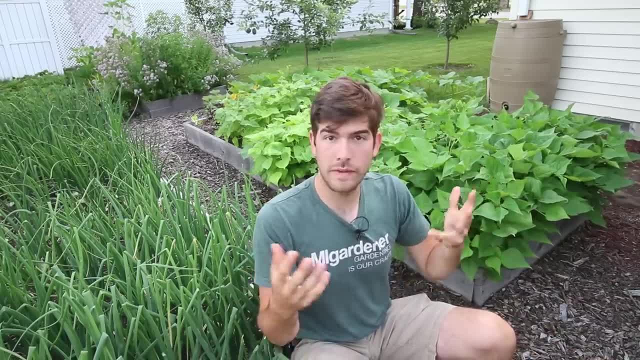 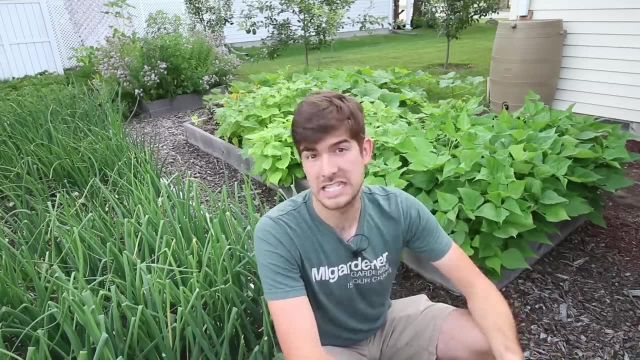 tend to ignore. They don't really notice until they become a problem, and then, when they do become a problem, they don't know how to get rid of the problem. And so these three ways are going to get rid of ants effectively and inexpensively. You know, I am not someone that wants to run to the 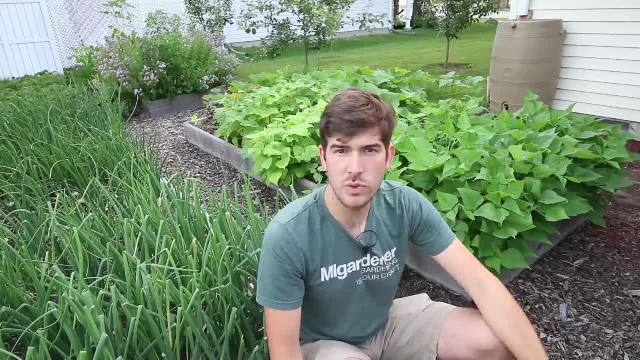 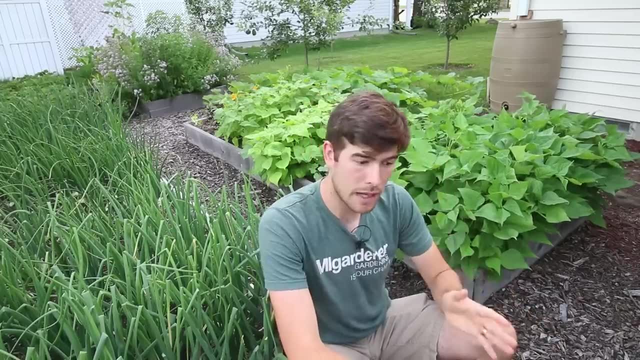 store and buy some super potent chemicals that I really don't feel safe even using around the garden, and also spending a ton of money on them. You know ants are something that are very easy to control. If you get up on them, you stay persistent with them, and you know, and you just 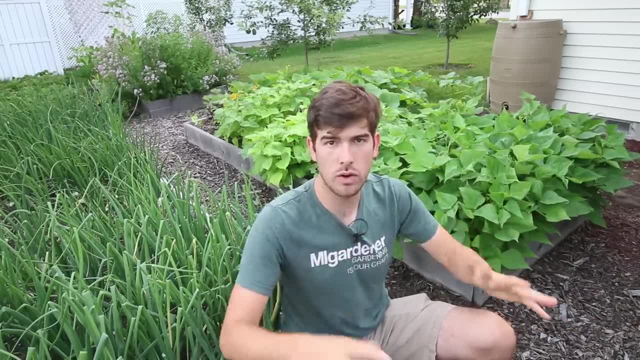 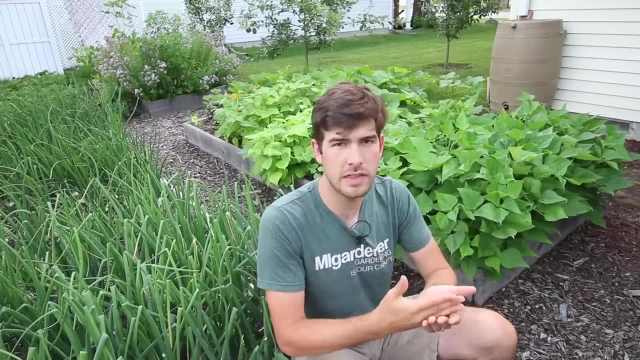 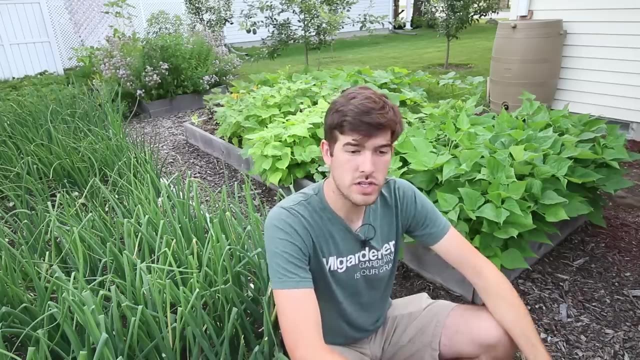 don't deviate from it. If you let them take hold, they will take hold. They're very aggressive with their colonization, And so what we have to do is just kind of nip it in the bud right away and make sure that we stay on it, because, like I said, they are very persistent, And if we do that, 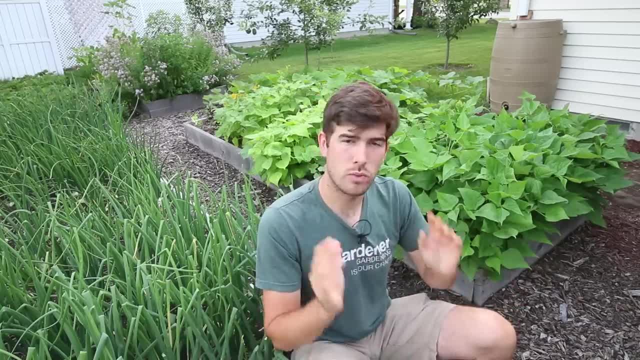 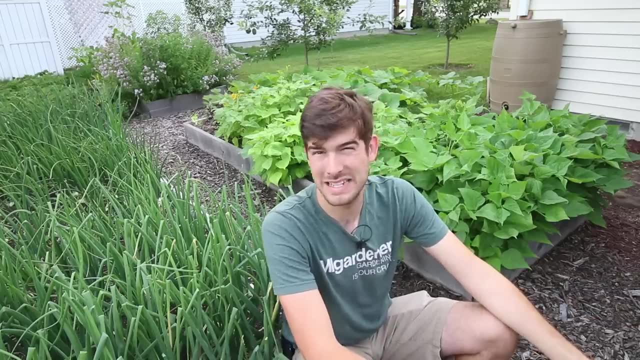 we can effectively control ants for pennies. So I really love these methods. I'm excited to talk about them. So ants are something we get asked, I'd say, at least 10 or 15 times a day. It's probably one of the most common questions we get, at least this time of year, because, you know, during spring, 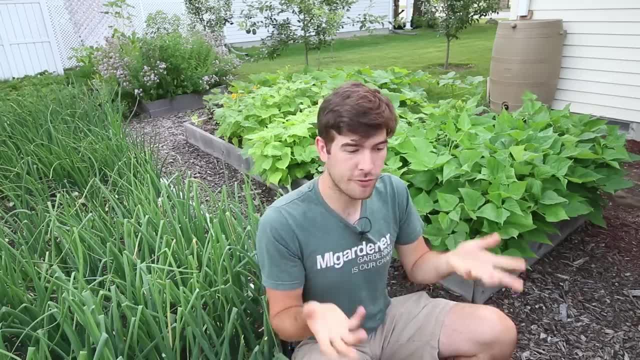 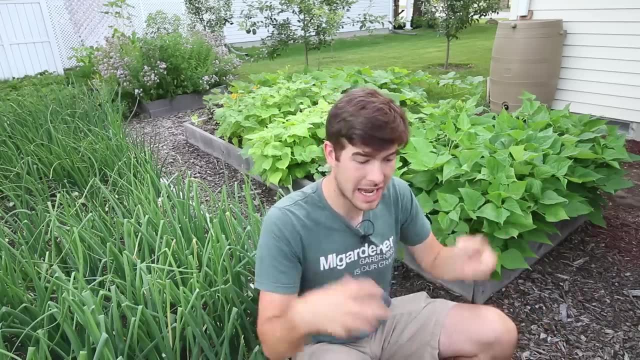 ants are not really evident, But during summer is when the food shortages become more evident and they become more aggressive and get ready to go dormant for the winter. So they're stockpiling all that food. They'll come into your house, They'll get into your garden, They'll start. 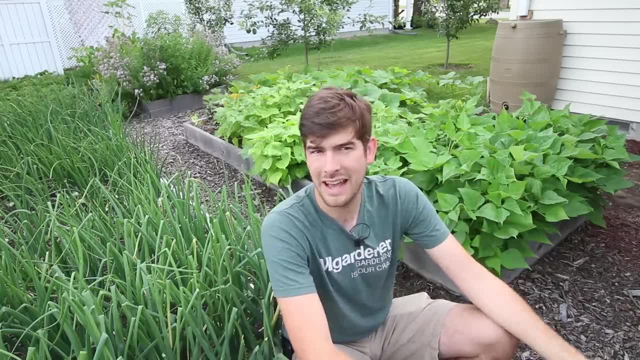 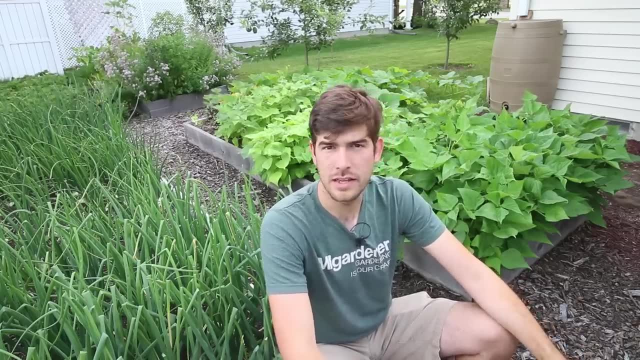 expanding their colonies, And it just becomes more of an obvious issue during the winter, In the heat of summer, which is why a lot of these questions start cropping up right around this time of year. The first thing I do want to talk about, though, are the problems that ants can pose You. 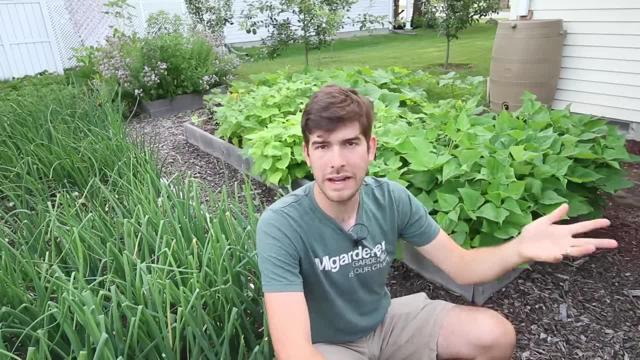 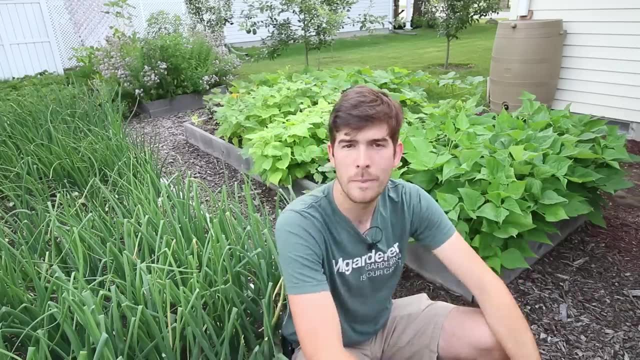 know, obviously they're a super nuisance in the house. They're, you know, they're annoying to have, you know, just even around the house in general, But in the garden specifically, which is kind of the topic of today's video, they can wreak a lot of havoc. We had ants that colonized our raised. 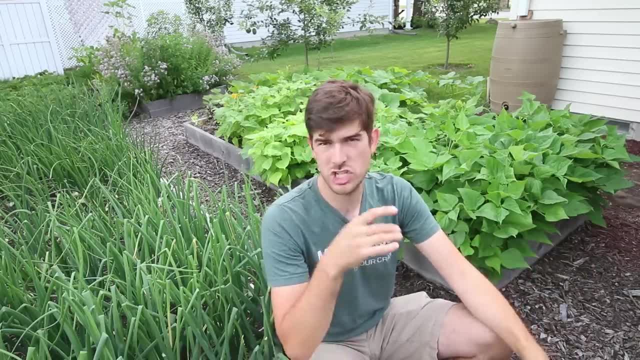 beds, And this is one of the worst problems you can have. You know, if an ant, if a stray ant, strolls around the house and they're not going to be able to get out of the house, they're not going to be able to get out of the house. 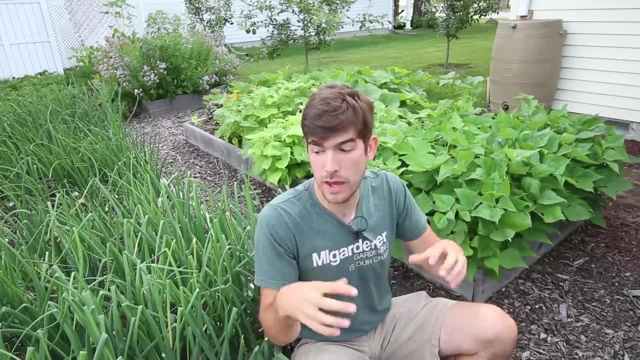 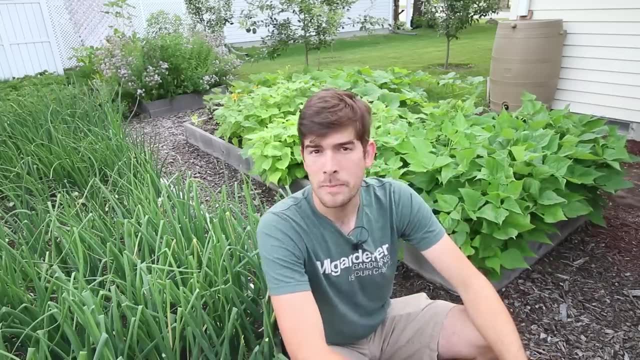 But when a colony of ants decides to take up residence in your raised bed or around your raised beds, that's when we need to take control and take, you know, you know- have a handle on the issue, Because they can really pose some serious problems. The first one is with seed germination. 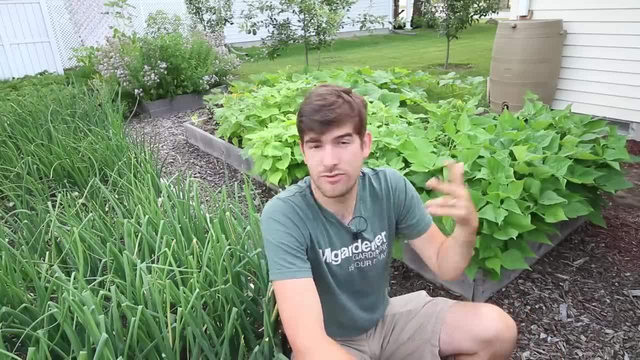 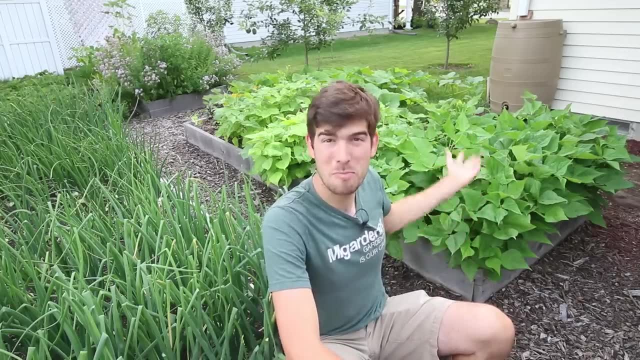 Seeds are rich in protein, fat and they're just a food source in general for ants. I've seen them carrying away lettuce seeds, grass seed even. they've even eaten beans seeds. And so you need to, you need to be able to control the ant problem, because if you put down, 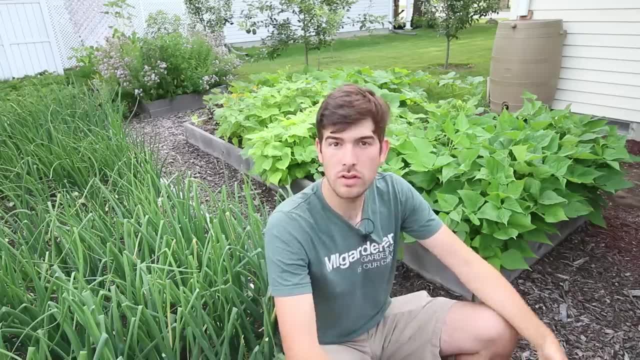 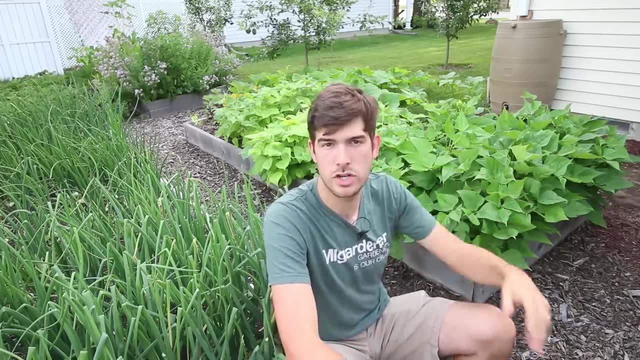 fresh seed. if you're starting anything from seed, they will consume that seed, They'll take it back, they'll stockpile it in their in their nest and then you'll have very spotty germination. The next problem is they over aerate the soil. When ants make a colony, they make tunnels throughout the 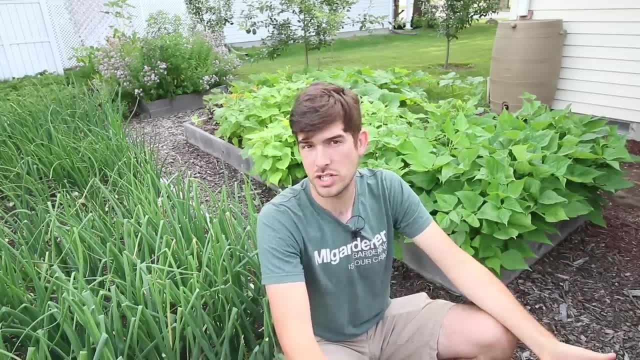 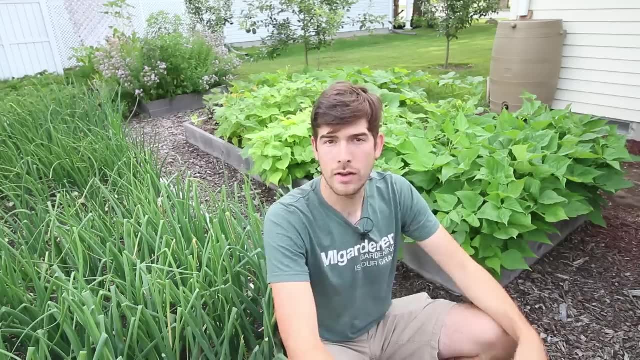 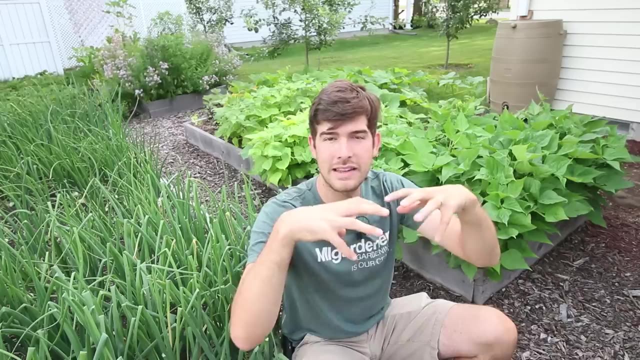 soil. These tunnels contain a huge amount of air that plants just are not used to, And the plant roots will actually touch those, those tunnels, and then turn, And what the problem is is that ants really love to make tunnels around plant roots because of the fact that the roots hold on to that soil and it prevents their colony. 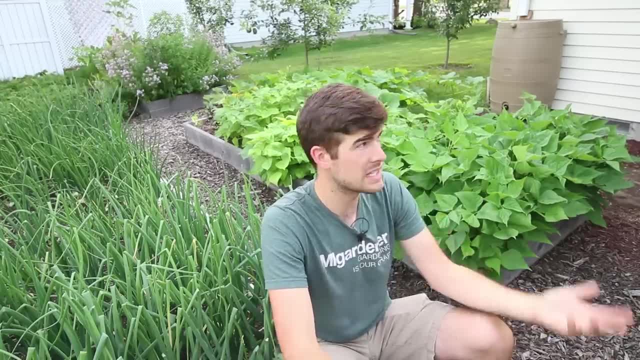 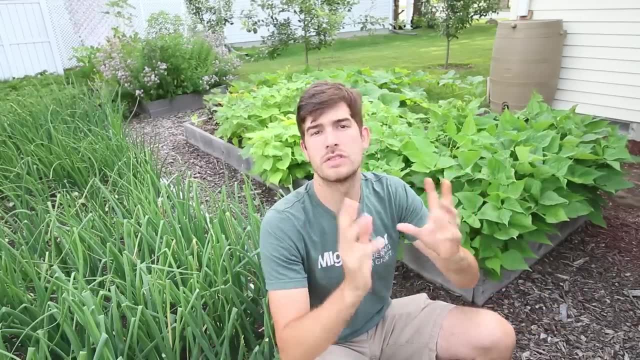 from collapsing in on itself, giving them a little more security. It's like you know, it's basically like the foundation of your house and you know the framework of your house. It helps kind of hold the house together, all those two by fours. So essentially the two by fours of the soil are plant. 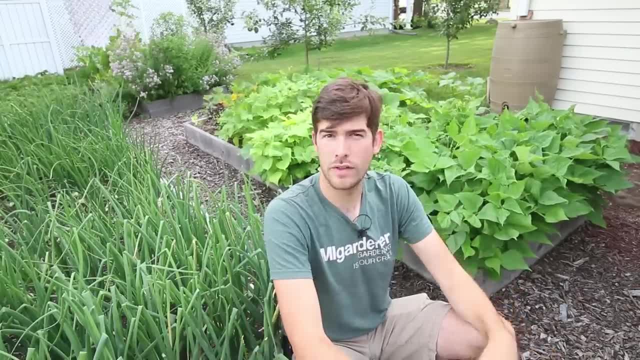 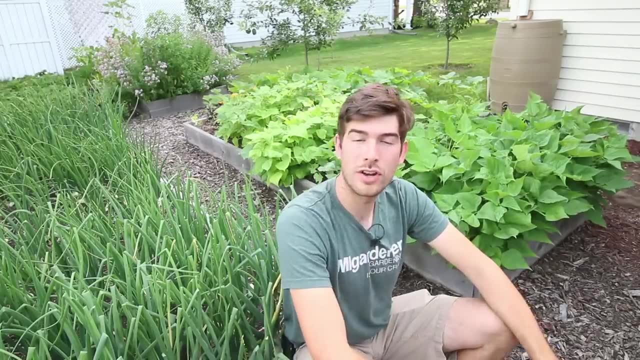 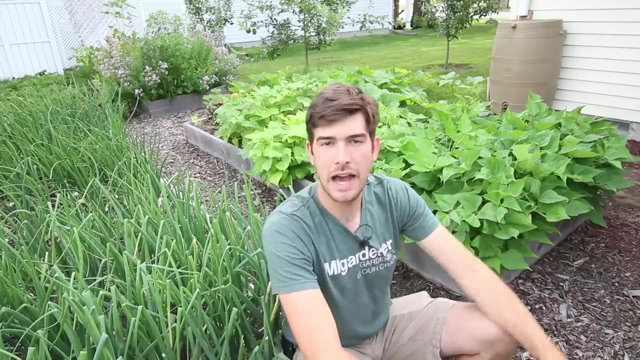 that's specifically why a lot of people will plant grass where there's erosion, because the roots hold on to that soil that will erode away. The third problem that ants pose in the garden are they bring aphids. Aphids are a soft bodied green insect that basically sucks the life out of your plants. They 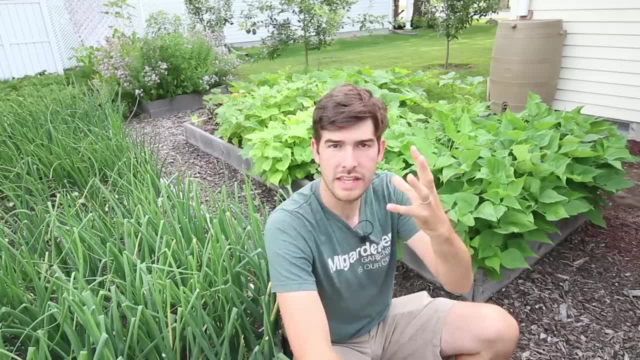 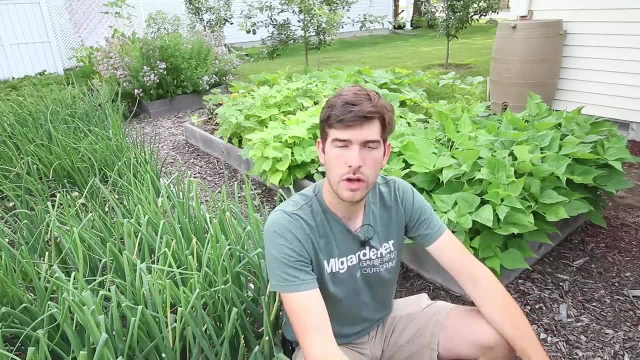 actually feed on the undersides of the leaves, sucking all the the sugars that the plant is creating through photosynthesis as a food source And then, as a byproduct, they excrete what's called honeydew. They take advantage of that sweet substance and the ants take advantage of that sweet substance as a 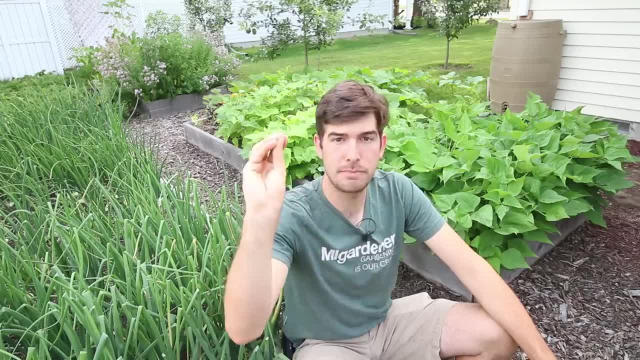 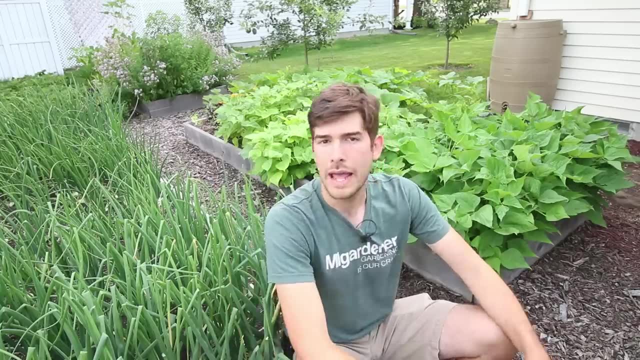 food source. So what they do is ants will carry aphids up to the plant, basically as a miner, and then they will. they will basically say, okay, I got you up to the plant, now you get me food, And this is a symbiotic relationship that the ants and the aphids have. However, it's a very negative thing. 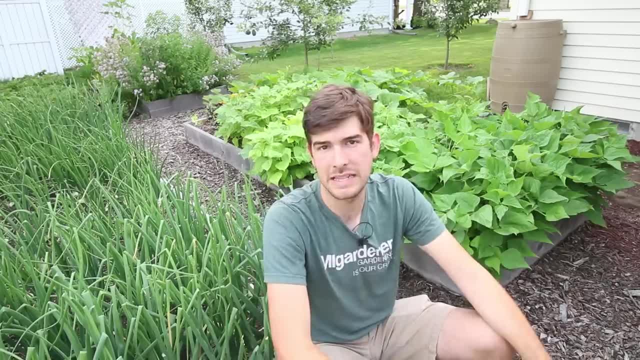 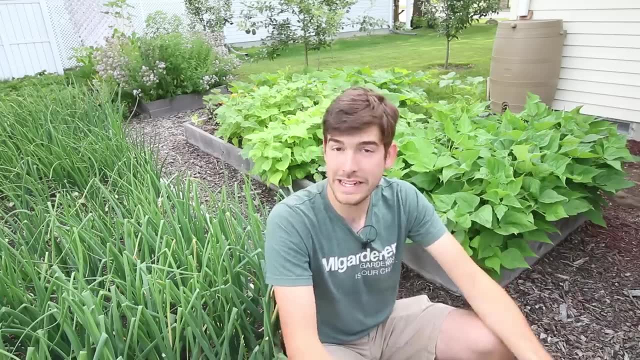 for your plants, because not only are the ants then encouraged to live near the plants, but they're also bringing aphids up which are killing your plants. So it's a double negative, and so that's why we need to take- we really need to take- care of ants in the garden. and the fourth and final reason why. 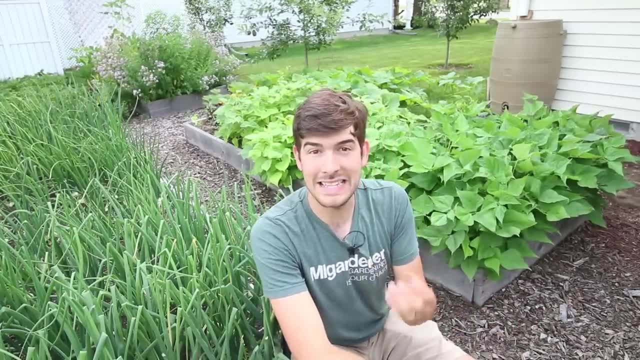 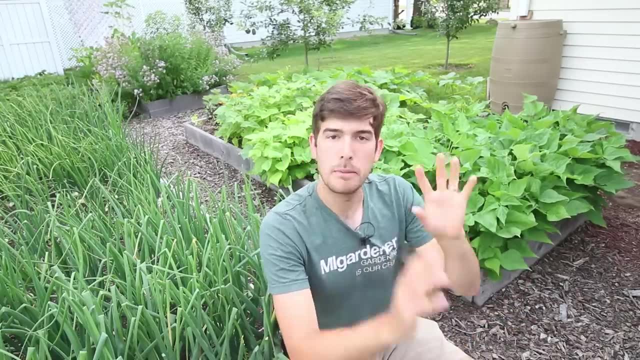 ants are not good in the garden, specifically, is because ants eat fungus. now you might be thinking yourself: well, luke, isn't that doing me a favor? i don't like blight. blight's a fungus, that's correct. blight is a fungus. powdery mildew is a fungus, however. however, there are good funguses and bad. 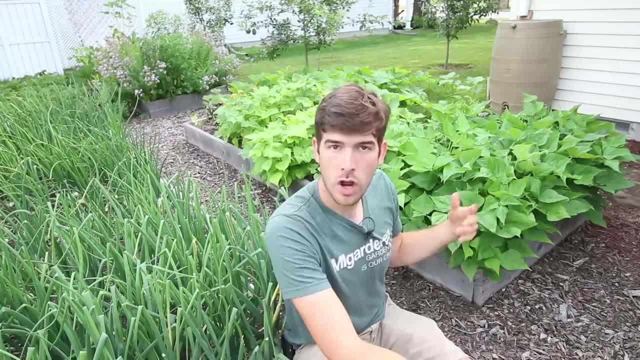 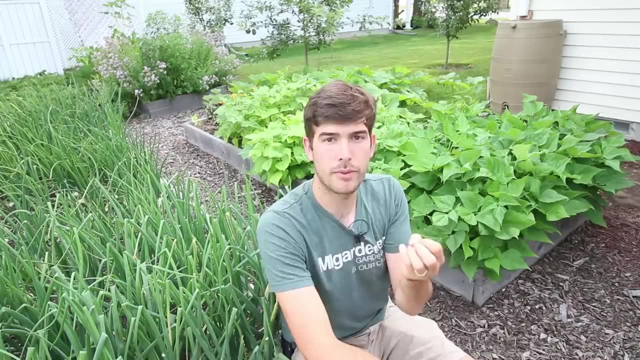 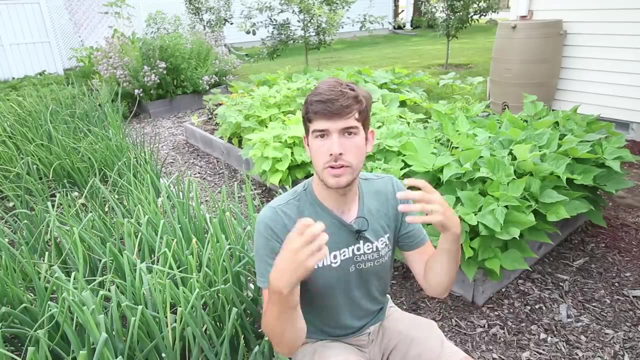 funguses, and the good funguses that you want are located in the garden, around your plant roots. it's called mycorrhizae. mycorrhizae is a is a fungus that attaches to plant roots and helps to mine minerals as well as increase the root system water resistance. uh. drought tolerance. 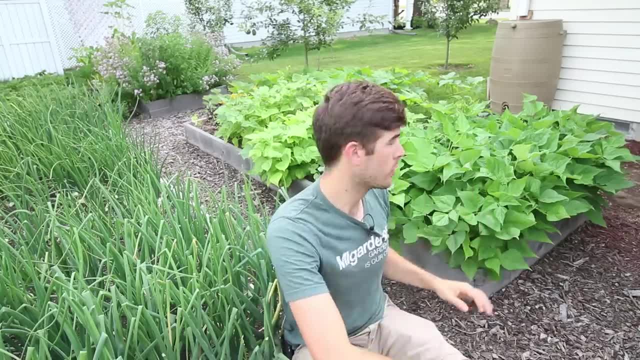 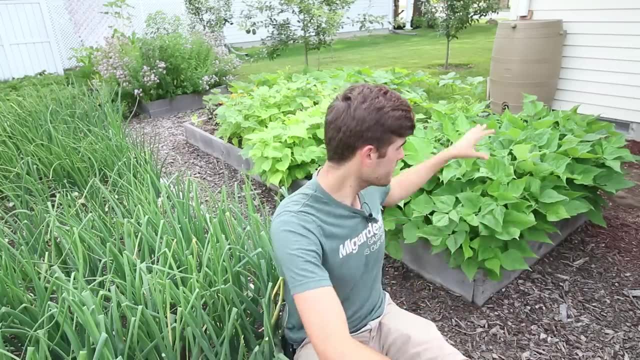 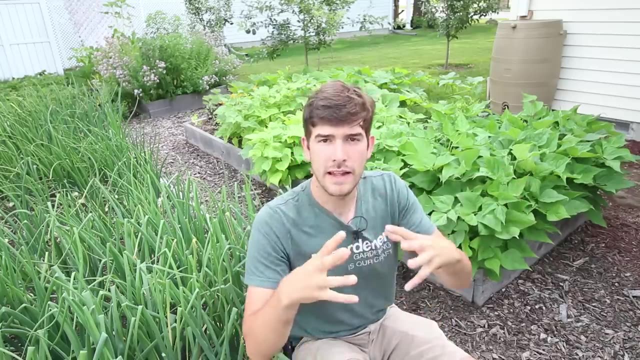 it is just an amazing thing to have attached to your plant roots. legumes, specifically, will form them naturally. they they attract the uh, the rhizobium bacteria, to the uh, to the root system of the, the beans. that's why, when you pull up your beans, you'll see these little balls. that's 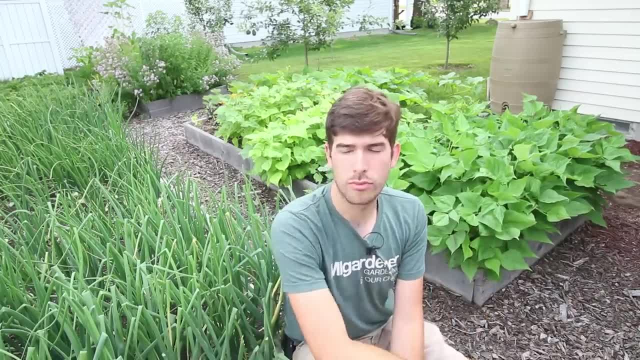 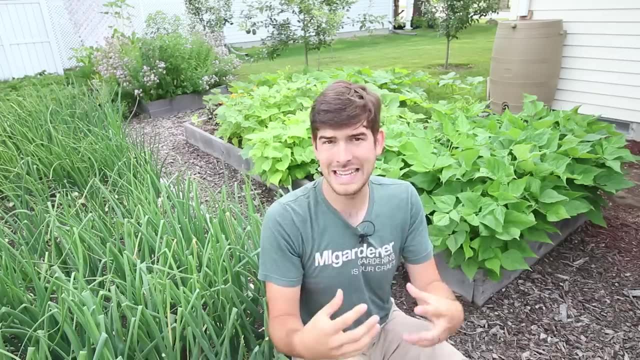 right up here. so you're just gonna just kind of grab that and put it down in a jar of water. just rhizobium that actually will form in nodules on the roots, and the thing is that it also is. if you inoculate your bed like we use trifecta plus it has it in there. but if you inoculate. 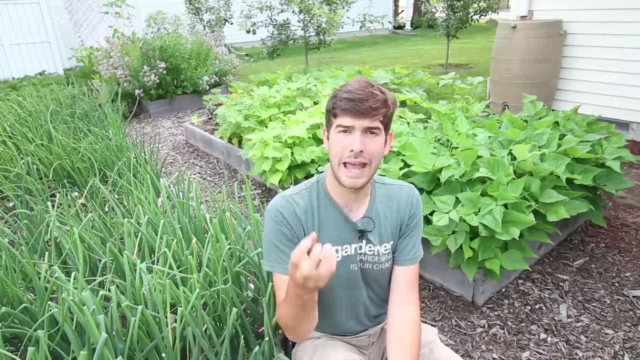 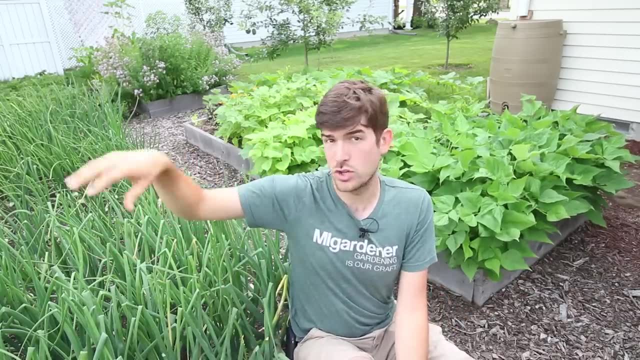 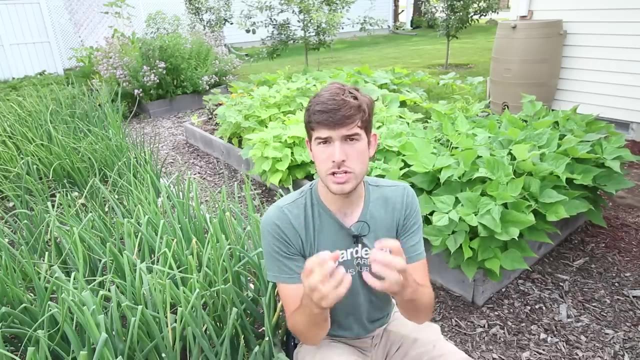 your bed or you use a really super good, rich organic matter compost that will have some, some mycorrhizae in there and that will attach to all of your plant roots- whether it's onions, zucchini, tomatoes, peppers, it really doesn't matter, it will actually attach to those plant. 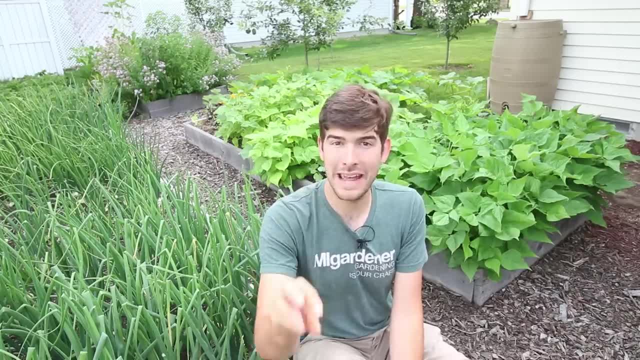 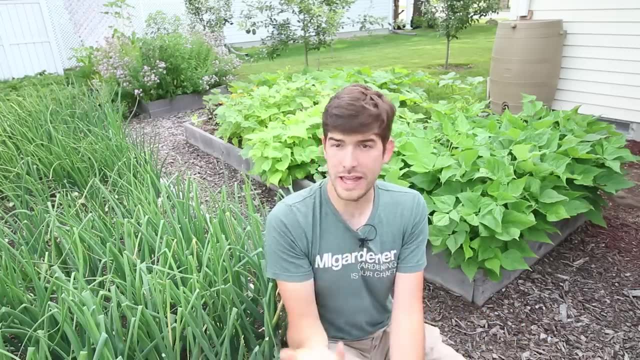 roots as well, and the issue is is that those ants will come in and actually feed off of that, off of that fungi. so you have reduced amount of fungus in your soil, which then reduces the amount of nutrients and and just health that your soil has. so those are four reasons why. 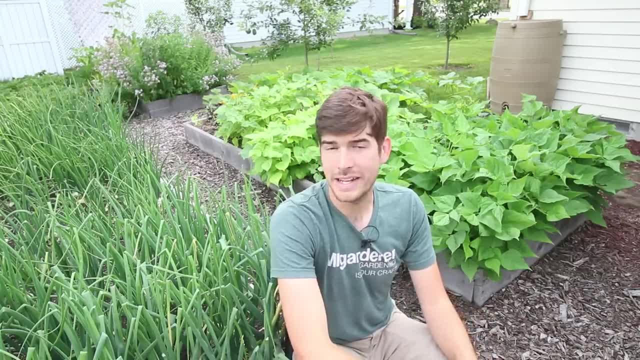 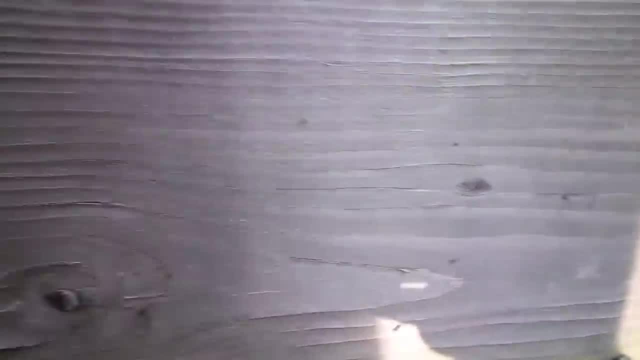 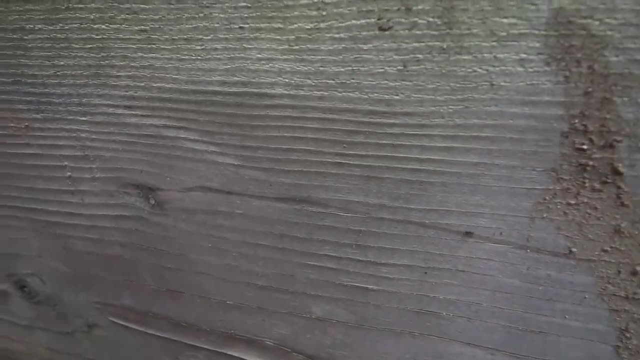 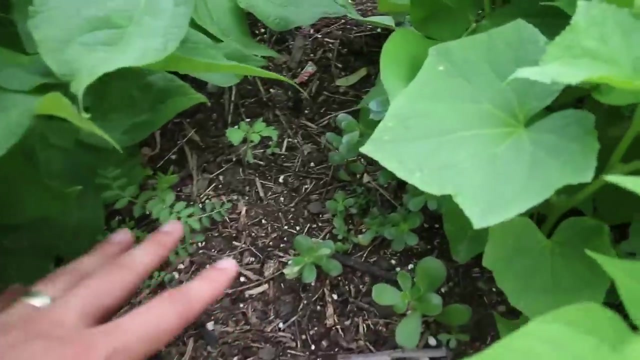 ants are a complete no-go in our garden and now we need to get rid of them. the first thing we need to do is locate their home. as you can see, we have a trail of ants, and the trail actually leads right up here into these dead patches. this dead patch is where they actually decided to make a colony. there's. 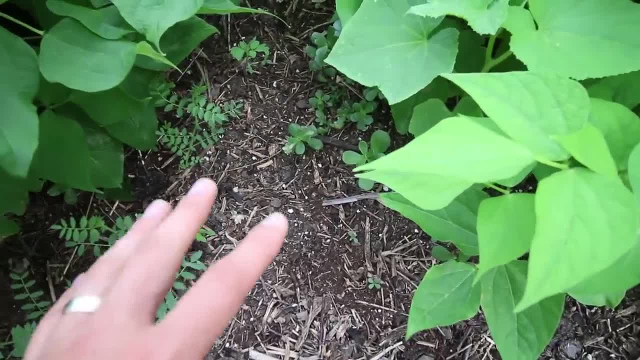 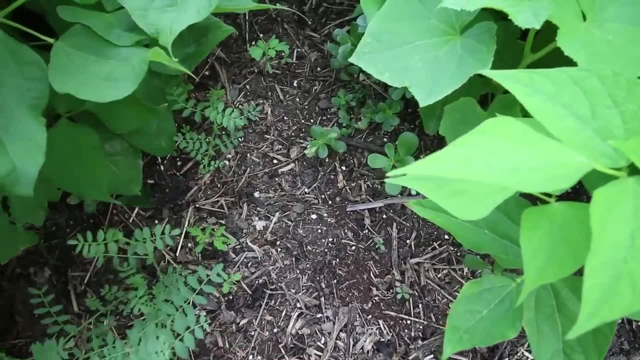 two colonies in this bed here, and what we have to do is, once we've located where they're coming from, the source, we need to treat this with our with our actual pest control methods. now, the reason why you can't get rid of these dead patches is because they don't have the 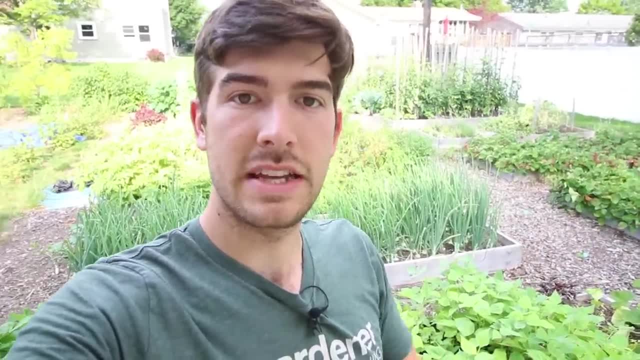 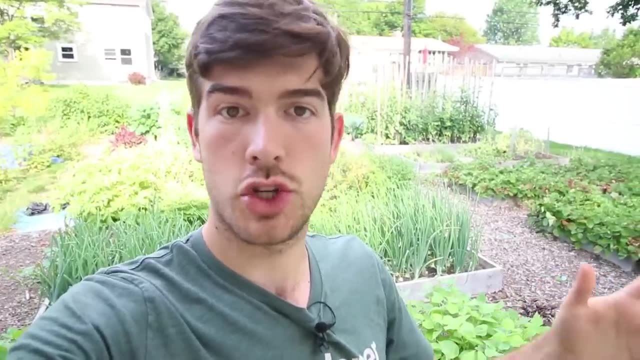 ability to feed off of that fungus. so you can't just spread these control methods willy-nilly is because they need to be treated at the source. if you spread them around willy-nilly they will not have an effect. if you just see ants in the garden and you see a trail of 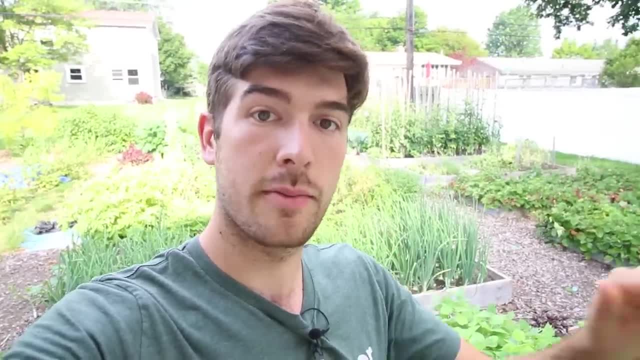 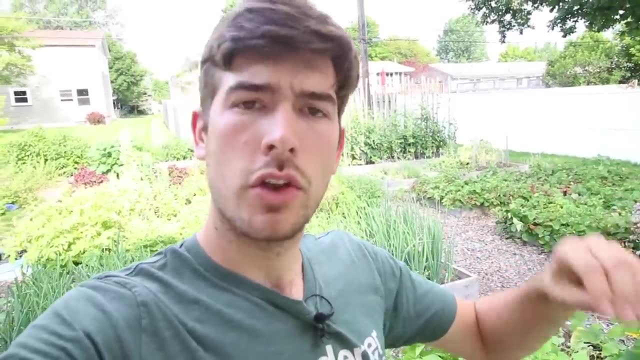 them. that's fine. you have to find the source. they're all coming from the source. that's what the trail is there for is. it's actually a pheromone trail that one ant will lay and it makes basically a train track. so what you have to do is you follow that train track. 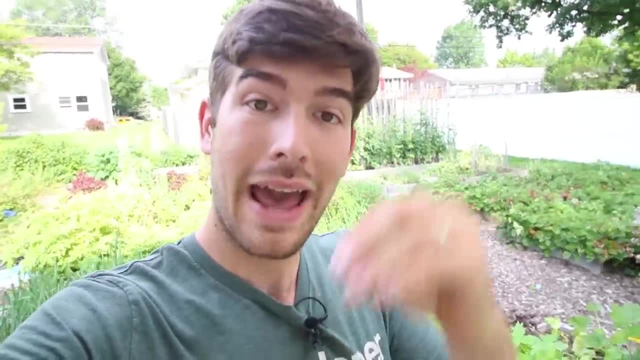 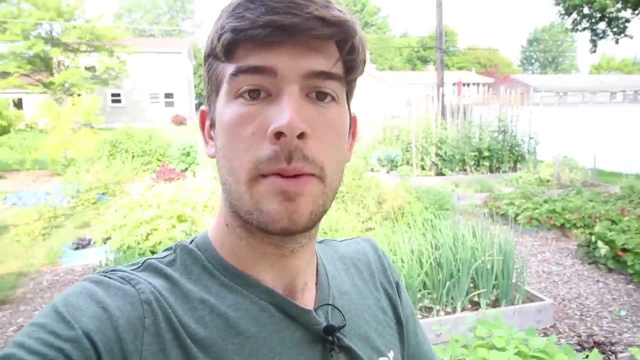 back to the source to find where the ants are coming from. you have to go at the source, because if you just treat the train track well, then you've done nothing. so the you know the whole purpose behind these three methods are essentially source treated, meaning they're going to be effective. the last thing you want to do is just waste time. 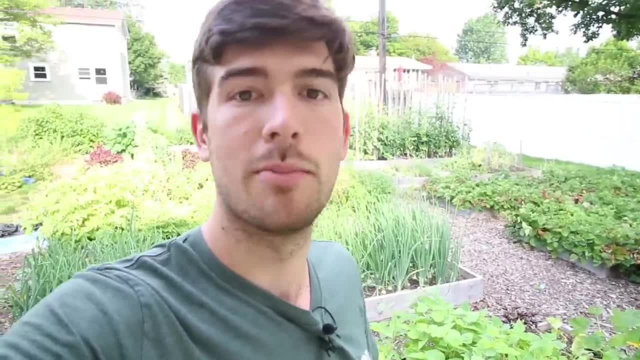 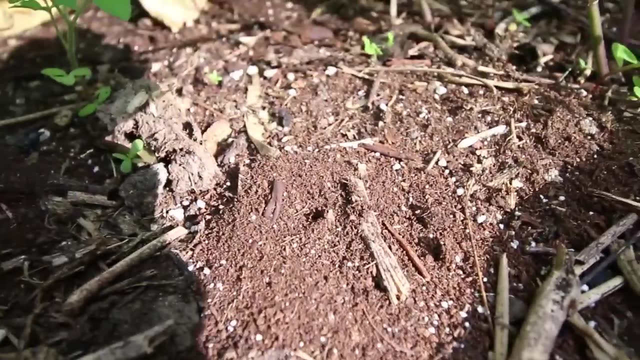 and materials by treating a problem that's not even really where the problem is located. so just keep that in mind, find the source and you'll fix the problem. and here we go. here it is. you can see there ant hill number one and here's ant hill number two. these are: 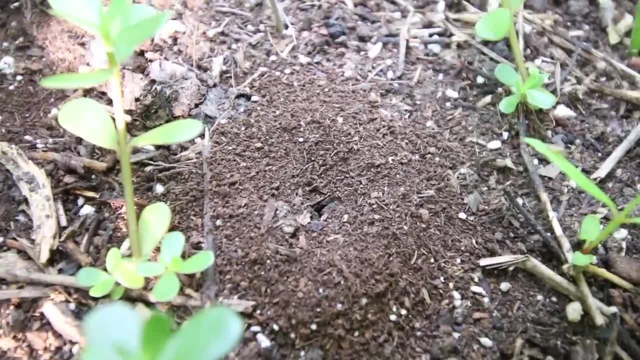 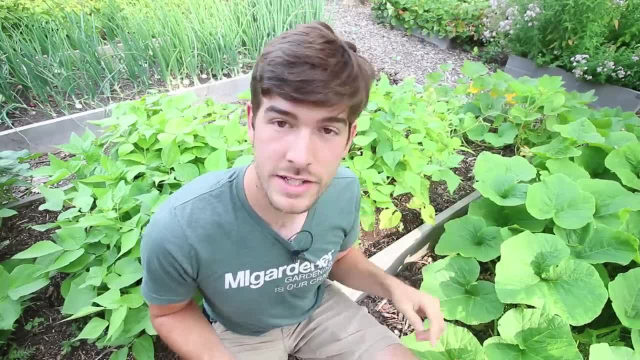 to go ahead, and I'm going to go ahead, and I'm going to go ahead, andIDO have to show you what that means. you really have to be careful. we're treating ant problem and you're sitting on the bed that has the ant problem. I might get some ants in your pants. 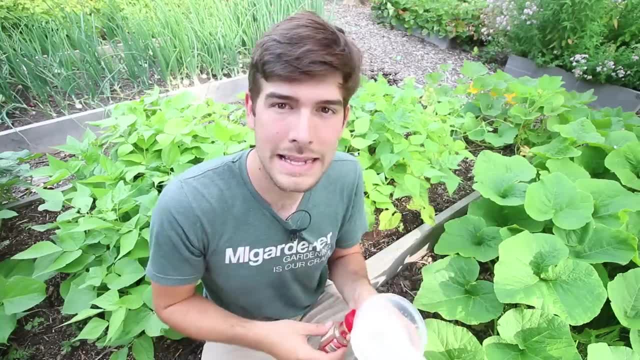 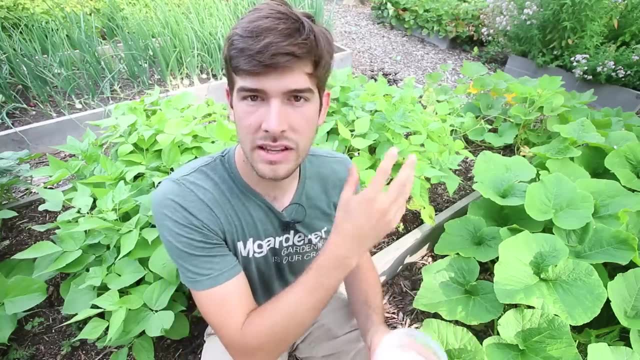 I had a couple crawling on my leg earlier. the first one is one that I don't have in my hands, and that's because it's the most readily available and it's actually your hose now. the issue is that this method is not really effective for in raised beds, because the fact 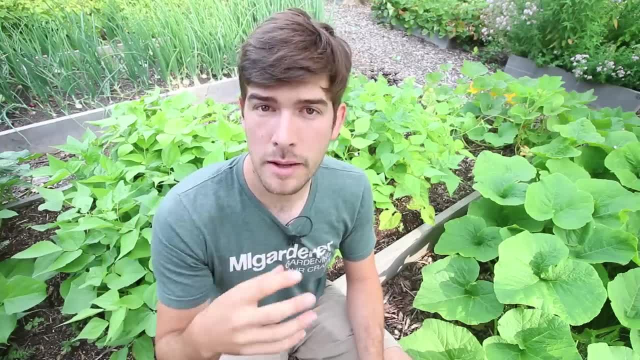 that we have plants here. it's called flooding. now, if you flood the bed or if you flood the source, they cannot. they cannot keep coming from ideas from- yeah, it's actuallyalling from, like a bird next to a ball, though I'll tell you what that does. well, the first method you 영out familiar down to some natural 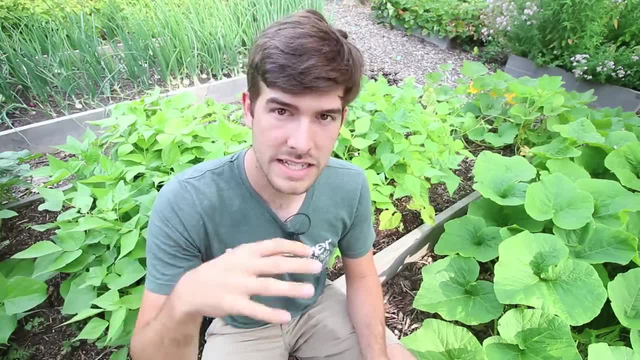 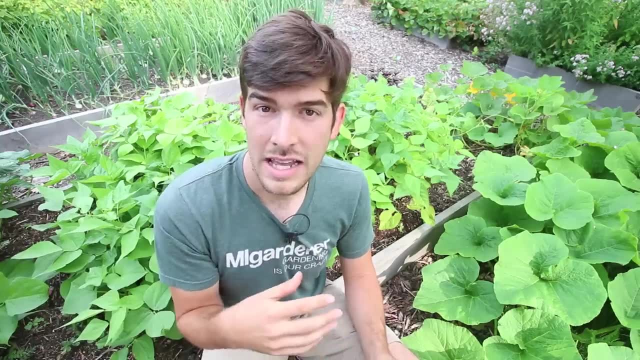 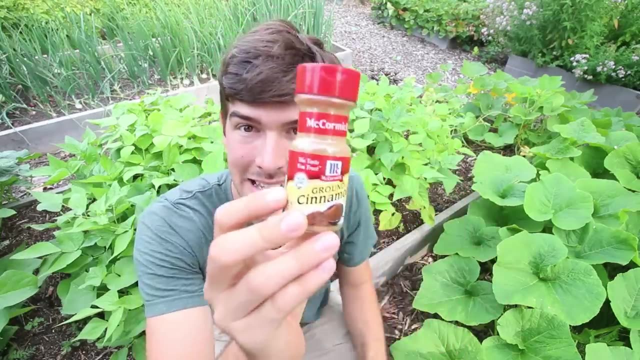 keep colonizing and so they end up moving. ants don't like places of low, basically low area, because that's where water settles, it floods their, their tunnels, it collapses their tunnels and also ants can't breathe, so they end up leaving to find higher ground. the second natural ant control method is cinnamon a. 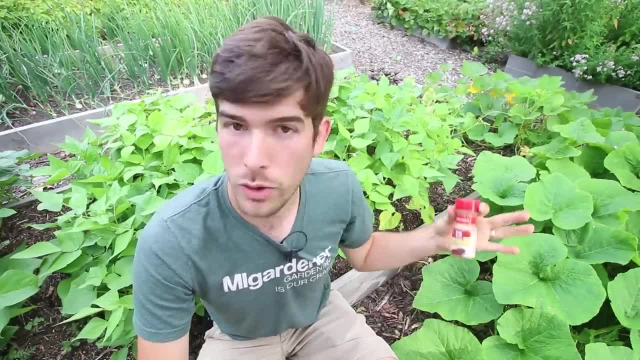 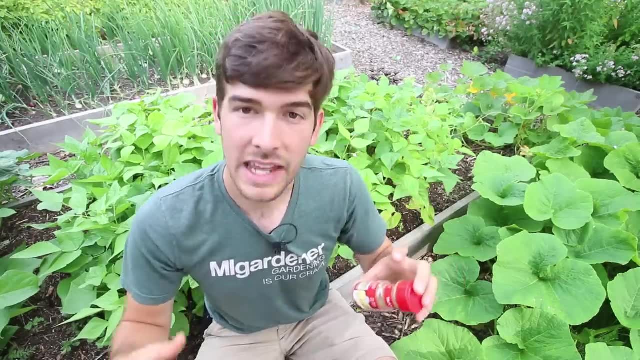 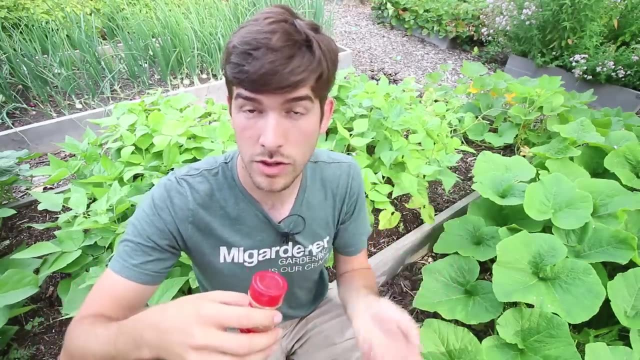 cinnamon is a super inexpensive spice you can get at any grocery store, even get a giant bottle of it if you really have a problem. but the thing with cinnamon is it's super effective if you have ants that are mining fungus. cinnamon is antifungal and so when you sprinkle it around the whole of the, you know the. 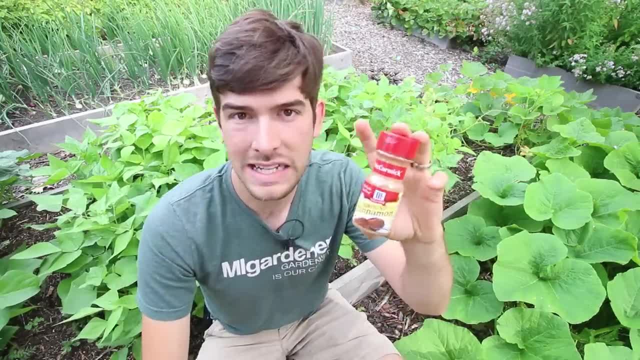 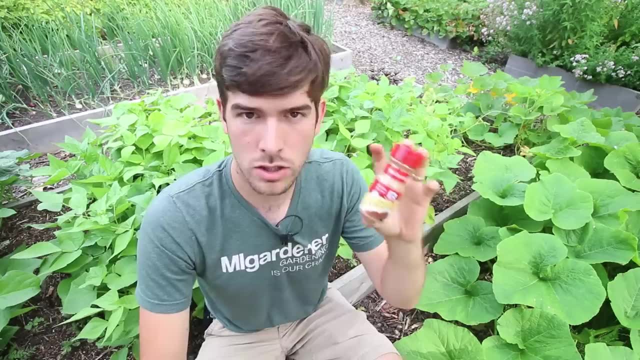 tunnel where the ants are coming and going essentially will kill any fungus in that area and they'll lose their food source, so they'll have to move now. this is something that works only if the ants are currently mining fungus. a lot of times, ants are out scavenging they're. you know they're trying to find dead. 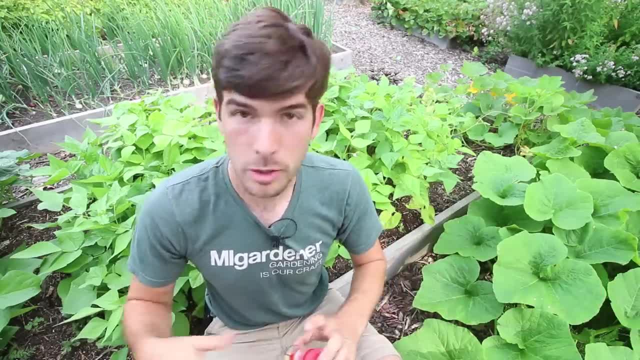 insects they're trying to find. you know honey from you know your beehive you're trying to find. you know honey from your beehive you're trying to find. you know honey from your beehive you're trying to find. you know honey from your beehive, or just a sugar source in general. 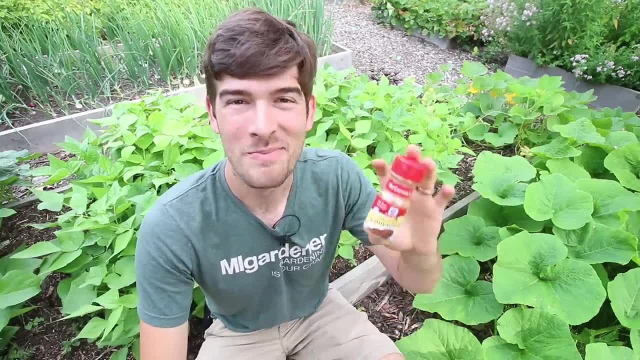 beehive or just a sugar source in general? beehive or just a sugar source in general? you know a lemonade, you left out two. you know a lemonade, you left out two. you know a lemonade you left out two weeks ago or something like that, but you. 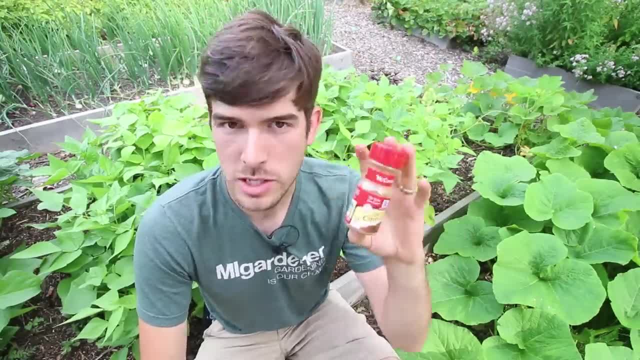 weeks ago or something like that, but you weeks ago or something like that. but you know this still is very effective. we know this still is very effective. we know this still is very effective. we found this does work. you have to use it. found this does work. you have to use it. 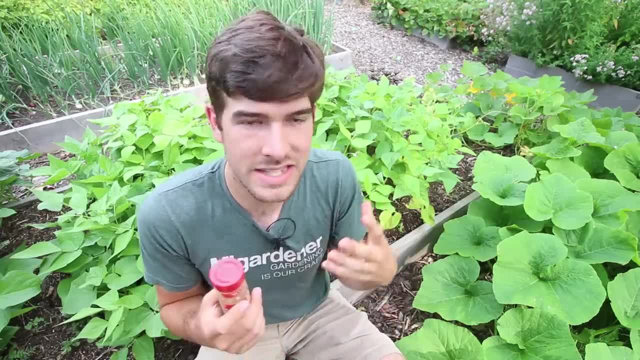 found this does work. you have to use it pretty copiously, and so I'll show you pretty copiously, and so I'll show you pretty copiously, and so I'll show you how much we use. and you know it's how much we use and you know it's. 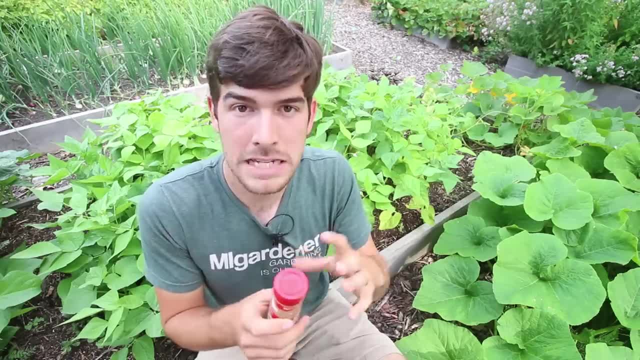 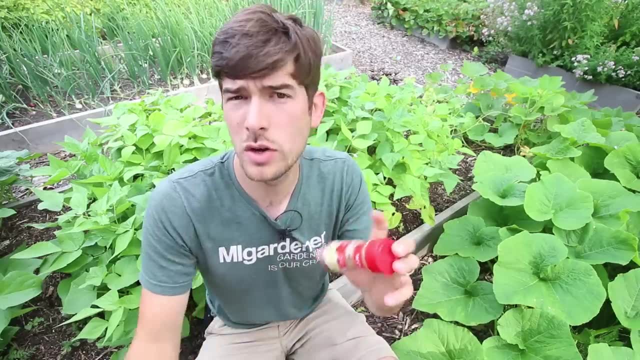 something that. try it, it might work. it's worked for us in the past, but it doesn't work all the time. it just depends on what the ants are doing at that current stage and uh, and you know, and you, you also have to make sure too that you don't have any rain. this, if it gets wet, really loses a lot of. 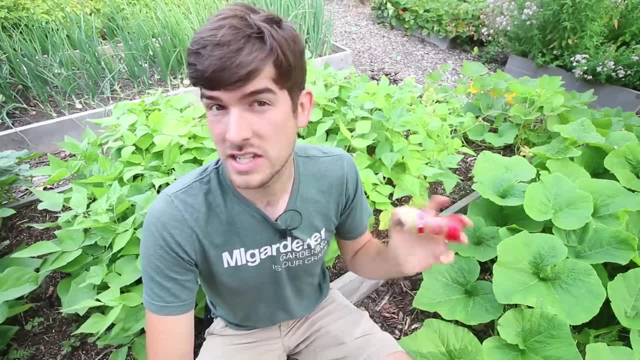 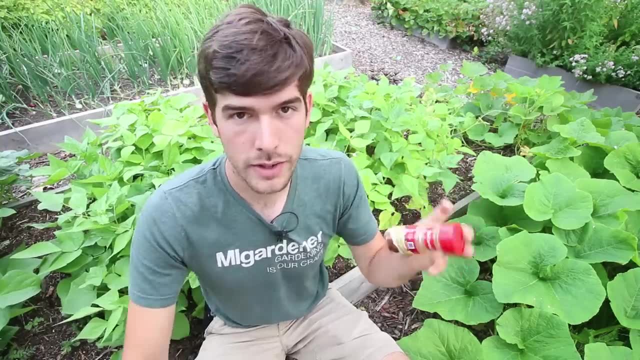 its potency. so during the dry season, the hot and dry season, i find this is the most effective uh than if you did it, like in springtime, when it rains a lot, because once it gets wet, it just pretty much washes away. so, um, let's use the uh, let's use the cinnamon now, so all we're going to. 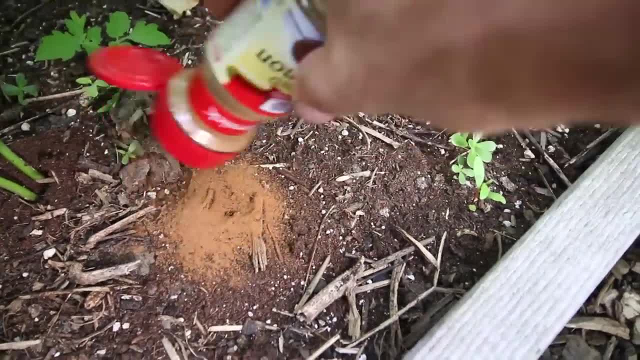 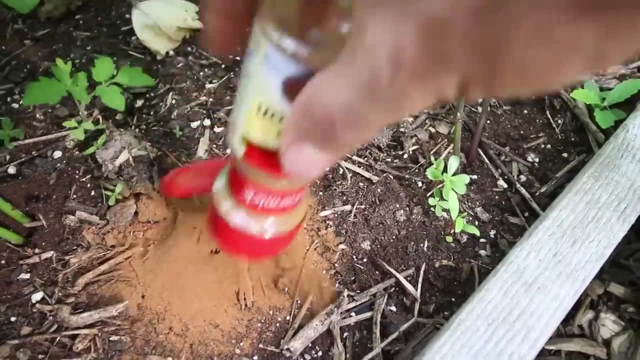 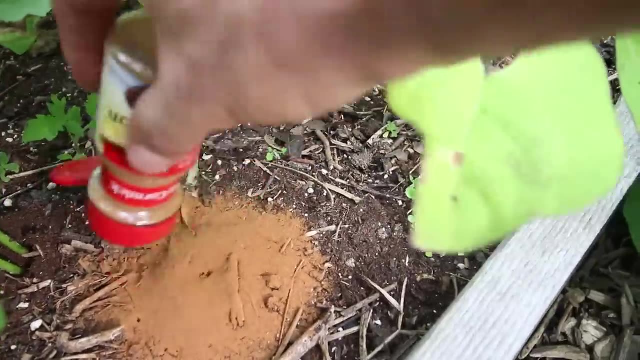 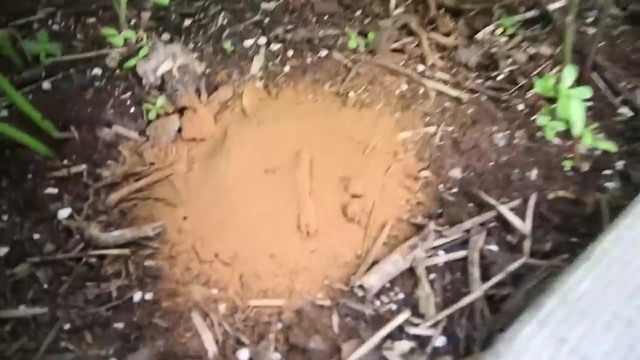 do is just take the cinnamon and use a copious amount of it. completely cover not only all the anthill but the surrounding area as well. nice thick layer of it. make sure you cover the hole up and that's all you have to do. and the final all-natural ant control method that we use. 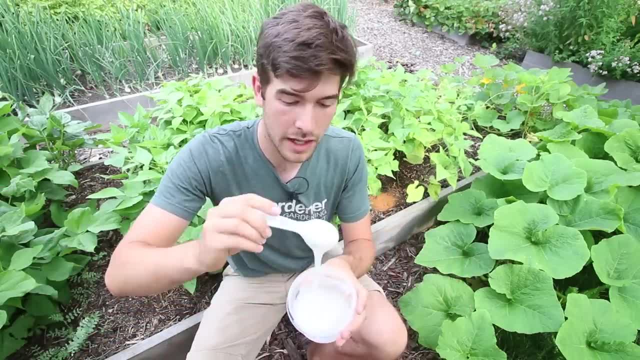 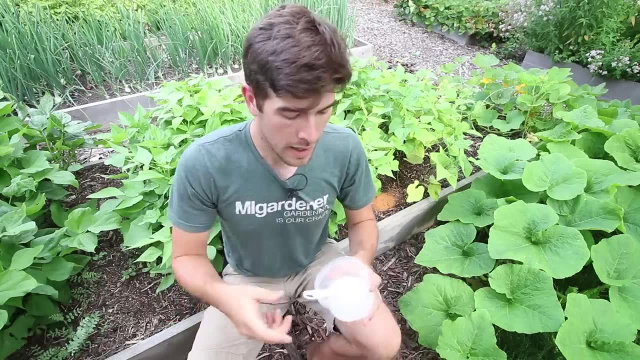 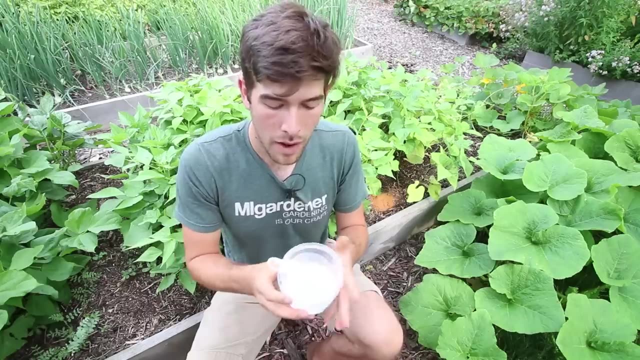 definitely the most effective of them all. one we go to if nothing else works is borax and sugar. now, borax is all natural. it's just boron and sodium and it's- uh commonly used as fabric softener. however, it's very effective at killing ants. however, a lot of times, people 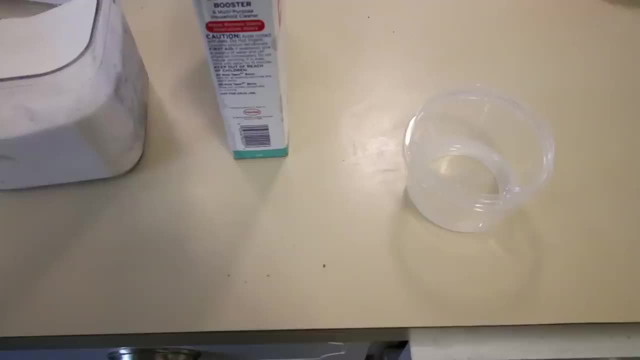 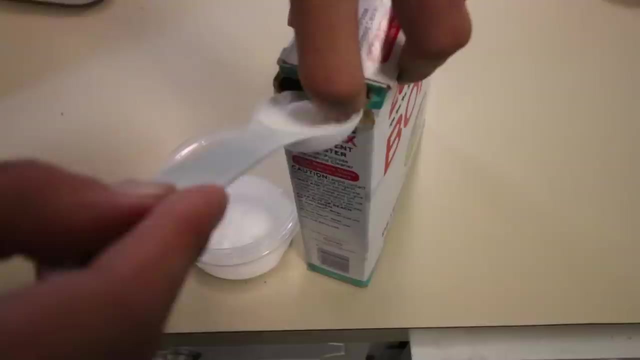 make? they make it too runny, they add too much water. what you want to do is: we made this up in our kitchen. it's super simple. all we did was we added one part sugar to one part borax. now the reason why you can't just leave it in its dry granular form is because 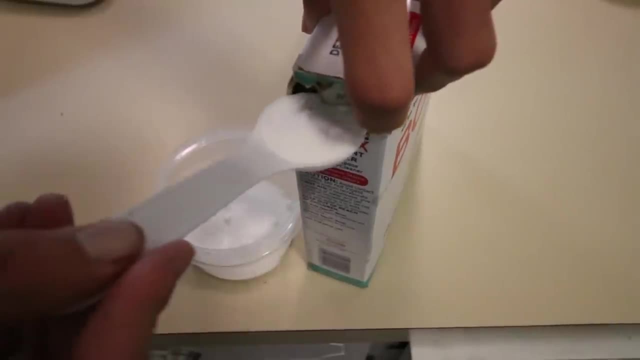 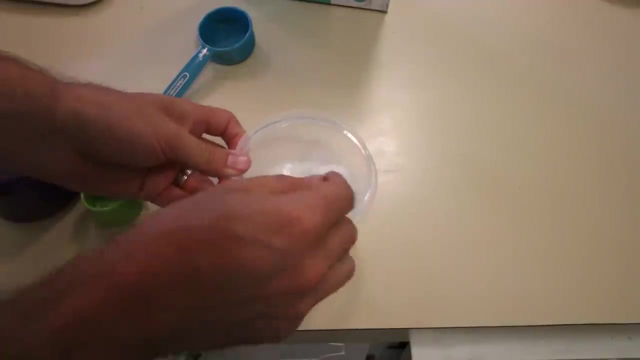 the ants will just pick out- they won't readily eat the borax- they'll just pick out the sugar and you'll just give them a food source. so what you want to do is add just enough water to make it a paste. once it is a paste, they can actually carry that. they can carry that paste back to. 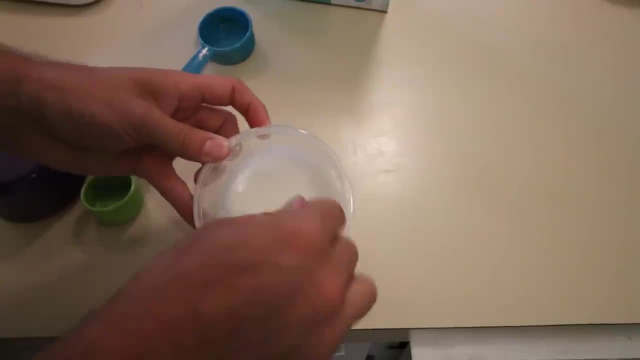 the anthill and feed the rest of the ants with it. so that's what we're going to do. next, we're going to add a little bit of borax to the anthill and feed the rest of the ants with it, if you make it too much. 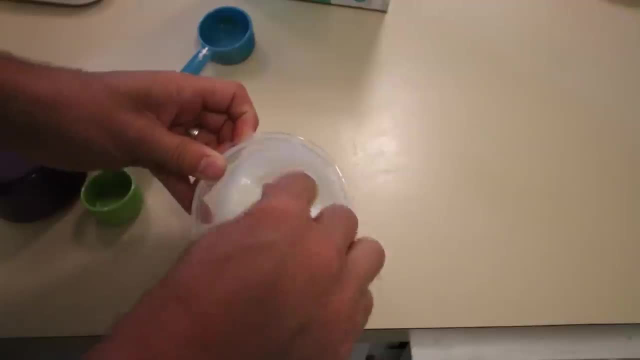 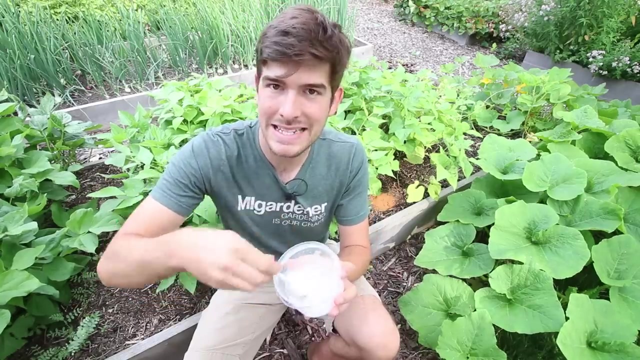 of a liquid. what can happen is they'll actually drink the liquid and it ends up killing them too quickly. they don't even make it back to the anthill in time, and so what we want to do is make it a paste, and it also helps if we apply it right at the source, because that way the ants are. 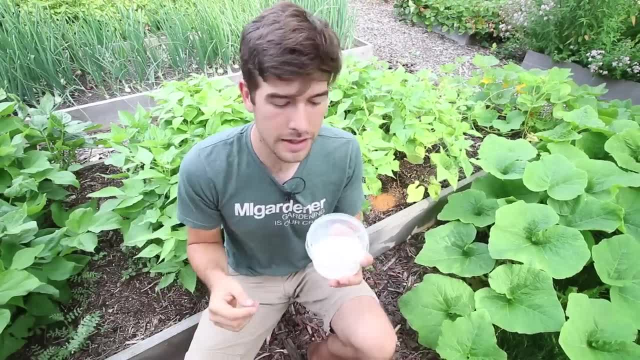 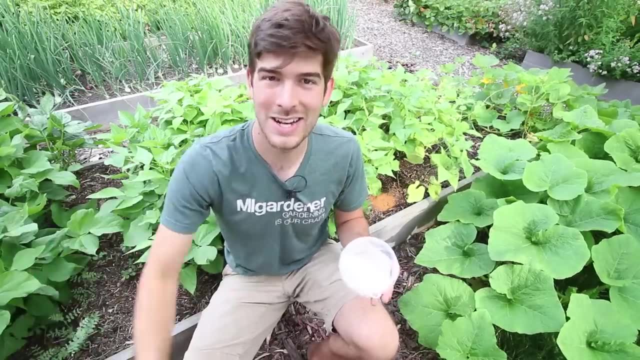 not carrying it a long distance, they're getting it and they're taking it right down and back into the colony rather than applying it 20, 30 feet away, where we see the ants, you see the kind of see those train tracks, those those ant trails. you can treat those ant trails and it will. 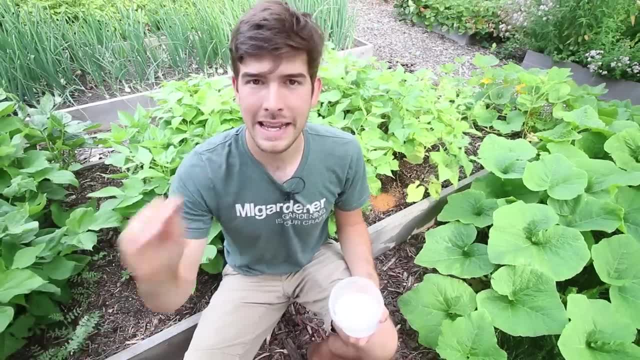 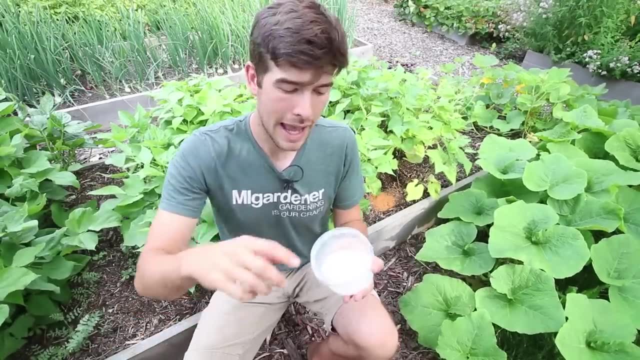 basically just bring more ants out there and the the colony will keep sending ants out to the sugar source and the answers won't make it back. so while it's effective, it's not nearly as effective and quick as putting it right at the source where the ants are going to swarm it, because ants are 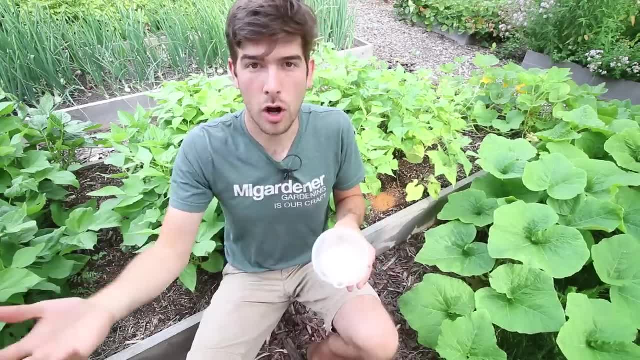 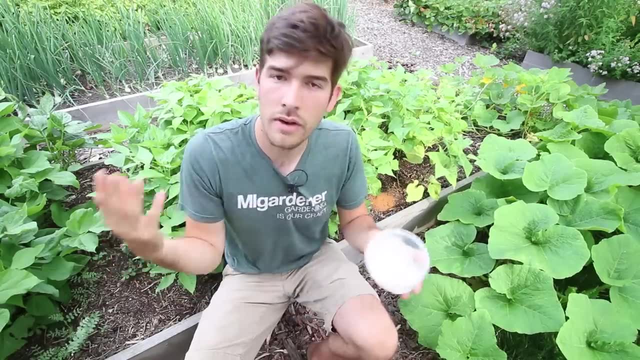 advantageous. they'll take advantage of a food source that's much closer rather than far away, and so feed them right at the source, this sugar and borax paste, and what they'll do is they'll take it, carry it down, feed the ants, hopefully feed the queen, because once you, once you feed, 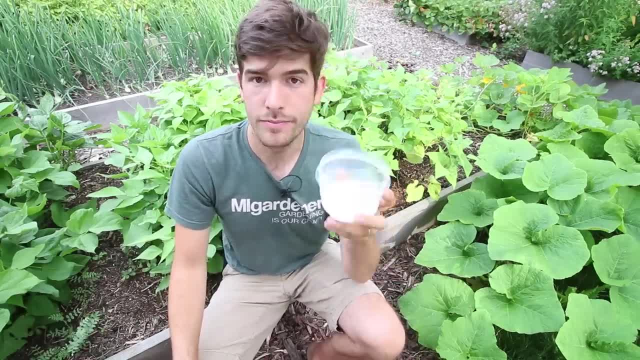 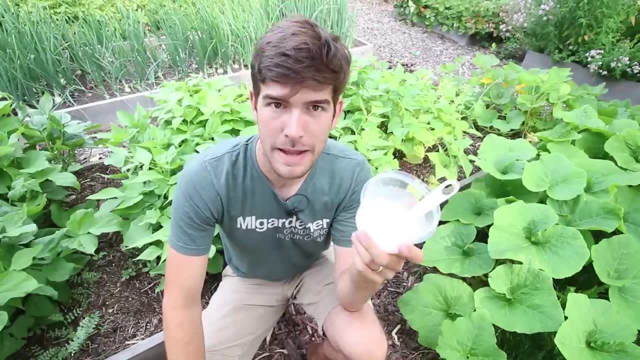 the queen. the queen dies, can't lay any more ants, so that's what we're going to do next. we're going to take the eggs and the, the colonies- pretty much toast. so this is a very effective method and it's very natural. so there you go, super inexpensive, and this might cost a couple pennies, the cinnamon. 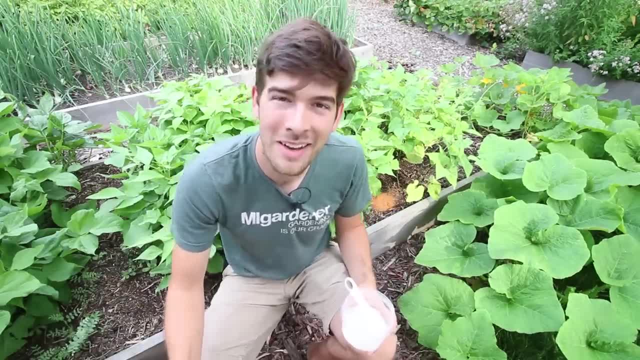 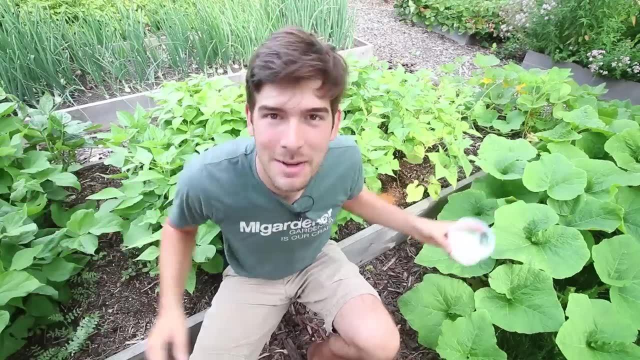 might cost a couple pennies and the water might cost a couple pennies, or free if you have well water, or a couple pennies if that well uses electricity. I know how you guys get. you guys are always hitting me with all the fine details I I got you this time, um. so either way, all three of 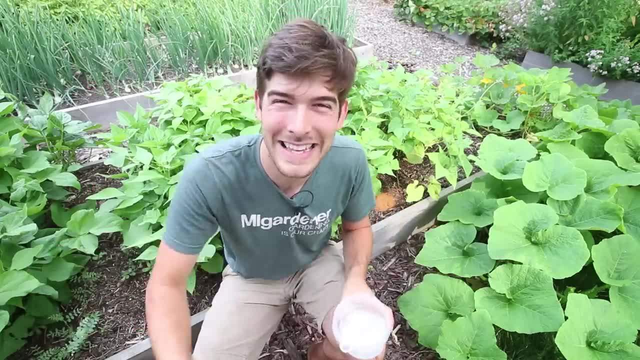 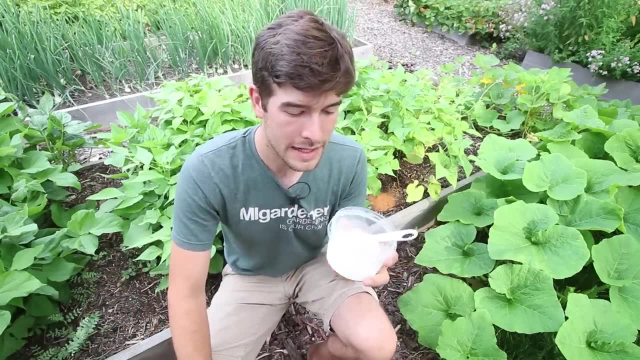 these methods are all natural and they only cost pennies, so I hope you guys enjoyed. I'm having fun in the garden today. I hope you guys are as well. I'm going to apply this to the beds now and, uh, what we're going to do is we're just going to put them. 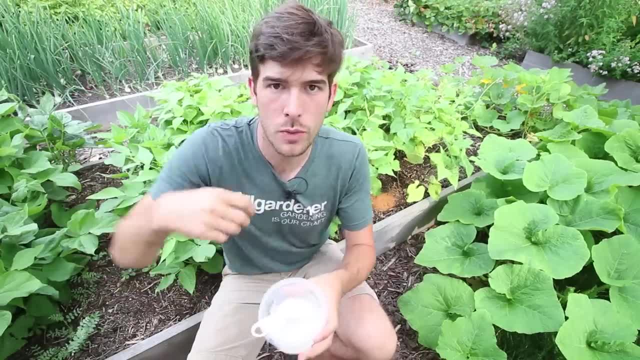 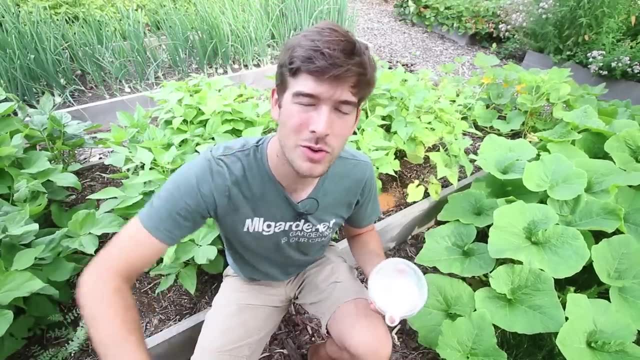 we're just going to put it, uh, in like a paste, just drizzle it right around the hole. they'll come out, they'll feed on it, they'll take it down. problem solved. so I hope you guys enjoy to help you learn something new. as always, this is Luke from the mi Gardener channel reminding you to subscribe if.